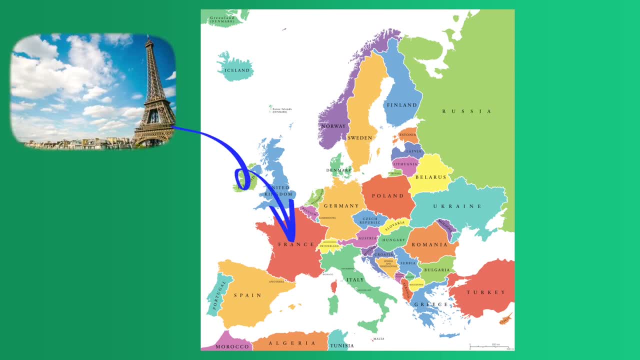 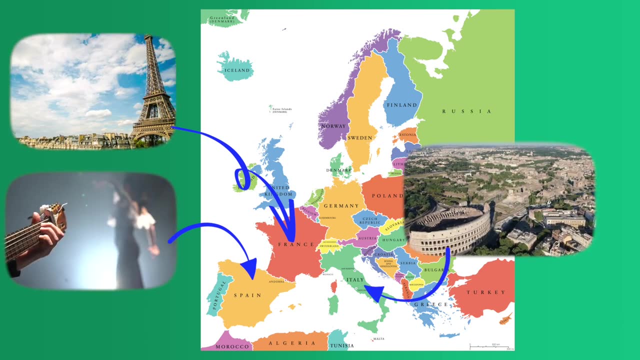 croissant while gazing at the Eiffel Tower in Paris, or perhaps you prefer taking in some flamenco in Madrid. Or you can take a historical tour of Rome and see the Parthenon, the Forum and the Colosseum. 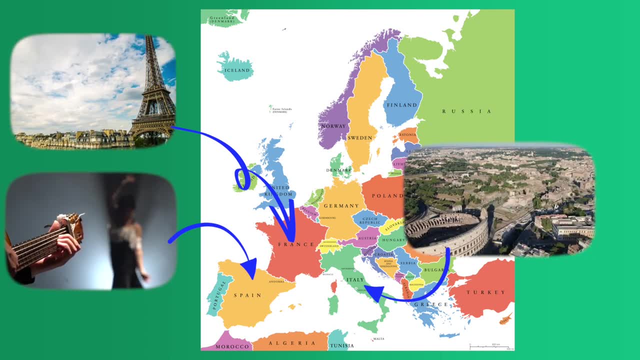 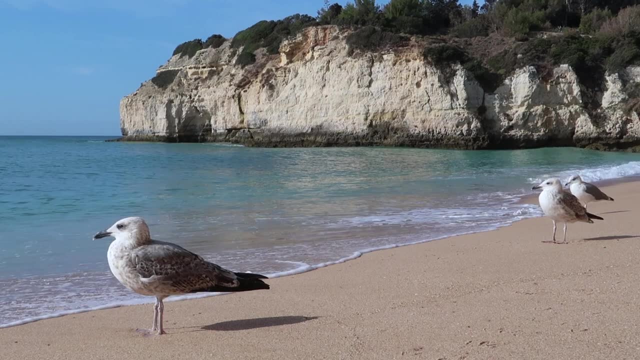 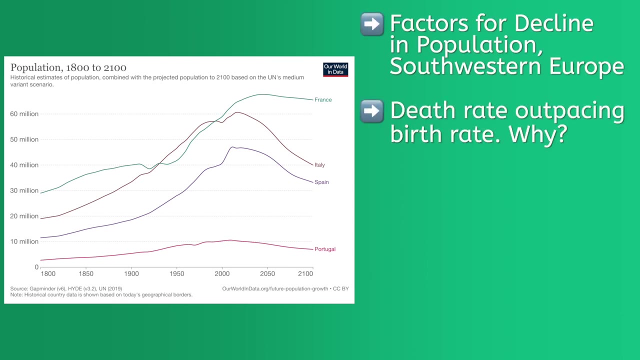 Yes, the cities of southwestern Europe have so much culture and history to offer. However, you may find the area a bit less crowded as years go by. The population in this region is projected to decline significantly by the year 2050.. The death rate is outpacing the birth rate and the cost of living in these. 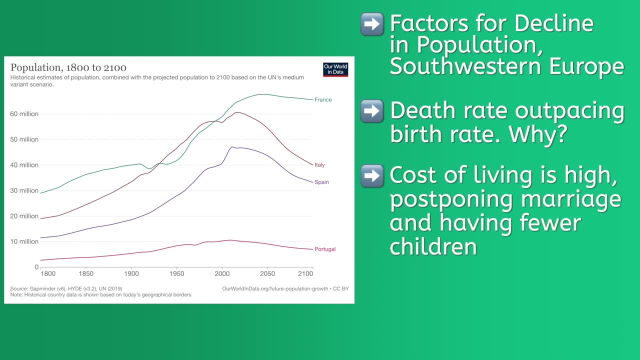 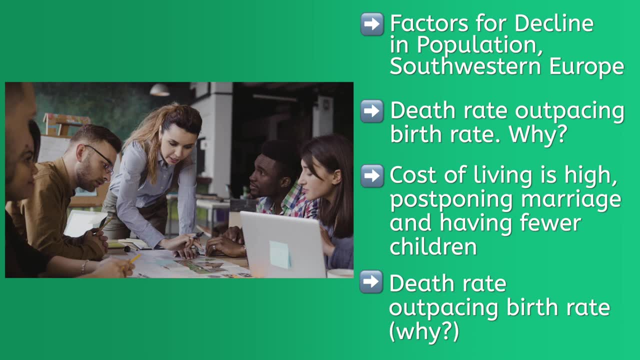 countries is fairly high compared to the income, So people are postponing marriage and having fewer children. Additionally, many are leaving for economic opportunities elsewhere. While these cities are cultural hubs, they're also a place for people to live, So if you're in a city, that's. 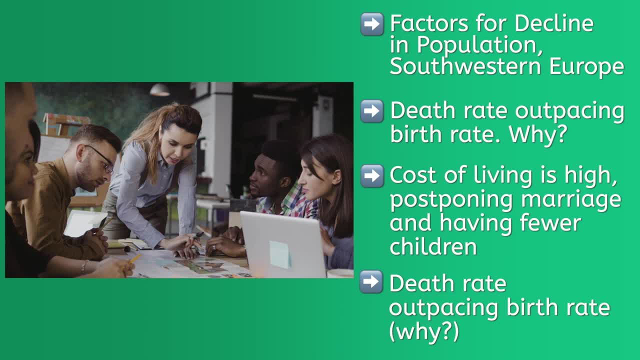 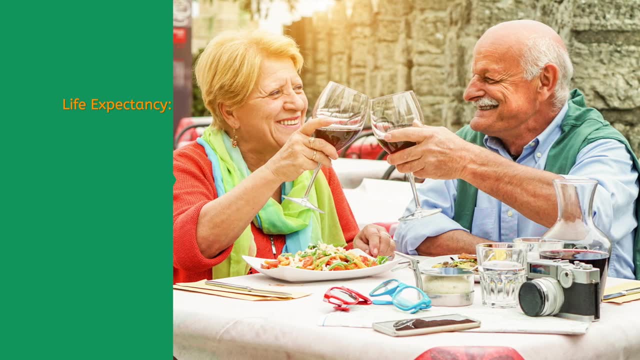 in the middle of Europe. there is greater earning potential elsewhere in Europe, But we'll get to the economy later. Those who do stay in southwestern Europe have plenty of time to enjoy it. The region has some of the longer life expectancies of the world. People in Italy and Spain enjoy nearly 84 years of life. 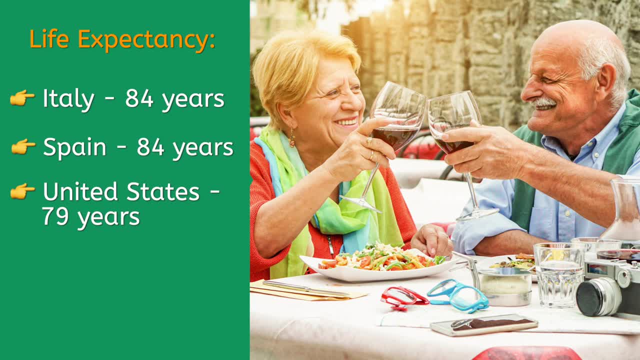 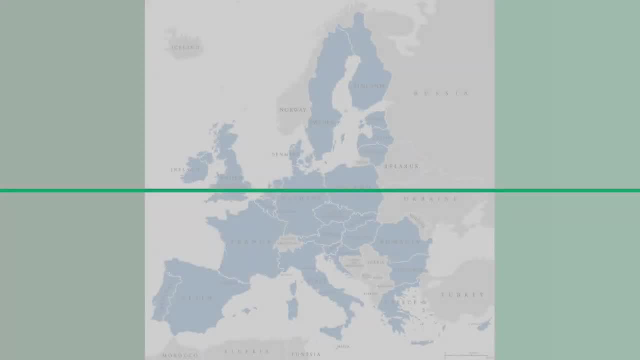 compared with 79 years in the US. Apparently, pasta and paella do the body good, Politics and Economy. Each of the core four countries are part of the European Union and all of the countries in the European Union are part of the European Union and all of the 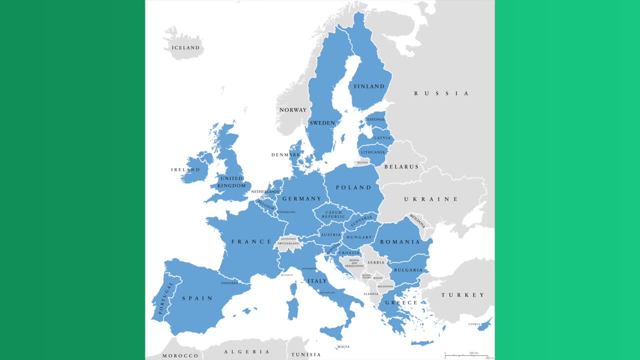 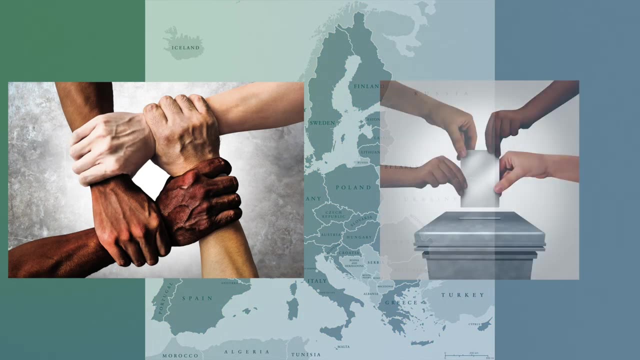 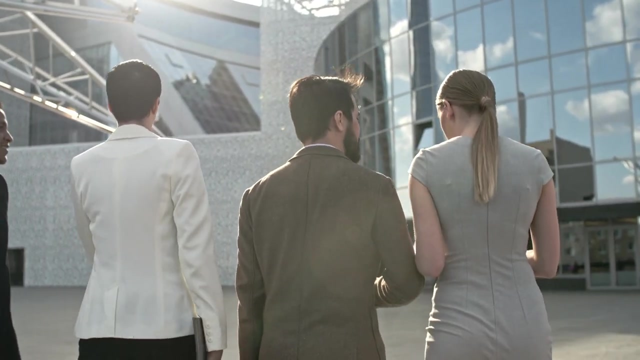 countries in the southwestern region rate highly on world measurements of political freedom. This means that, in general, their citizens are not denied basic human rights and they are able to participate in the democratic process. The GDP in southwestern Europe is high compared to the world's average, but lags behind the northern countries in western Europe. 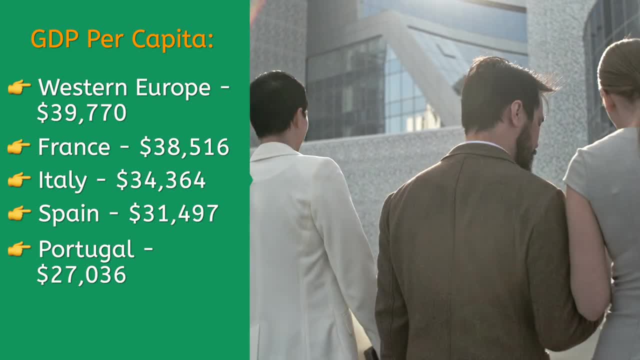 On average, all of western Europe's GDP per capita was $39,770 in 2019.. Each of the core four fell below the average. On average, all of western Europe's GDP per capita was $39,770 in 2019.. Each of the core four fell below the average. 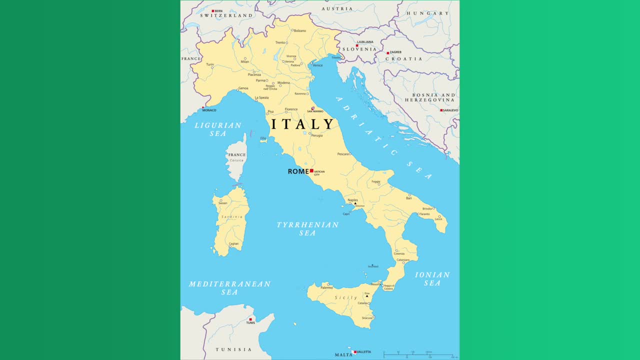 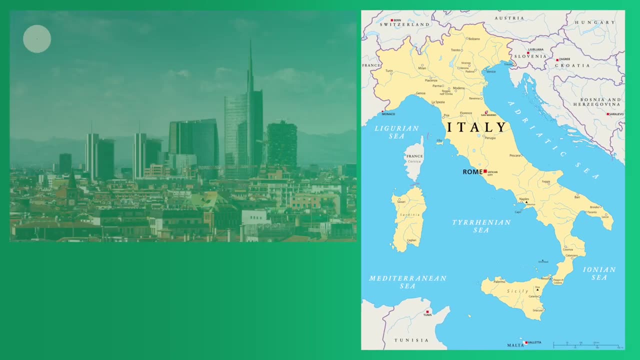 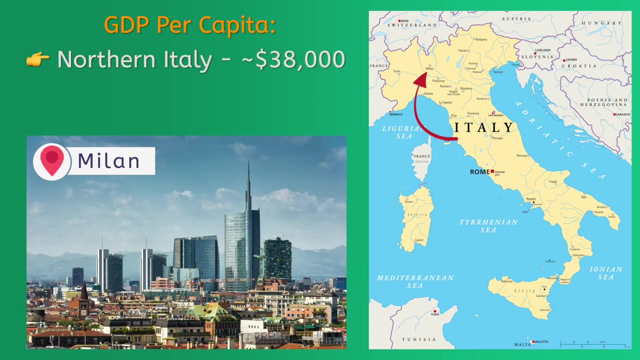 While there is a GDP per capita gap between northern and southern Europe, there is a similar gap even within southern European countries. Northern Italy, led by the city of Milan, is an industrial powerhouse and center of fashion design. In 2016,, northern Italy's GDP per capita was about $38,000, compared to $20,000 in agrarian southern. 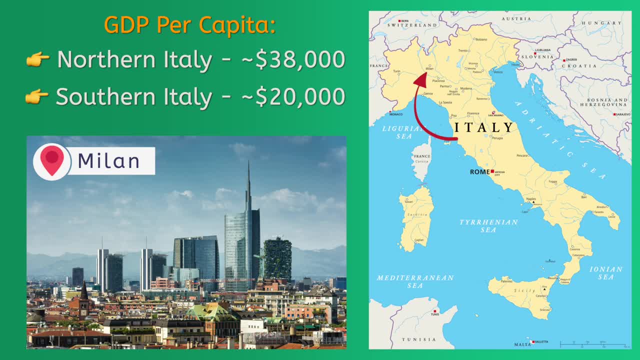 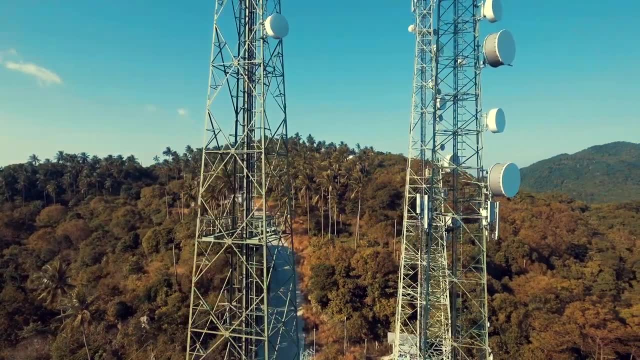 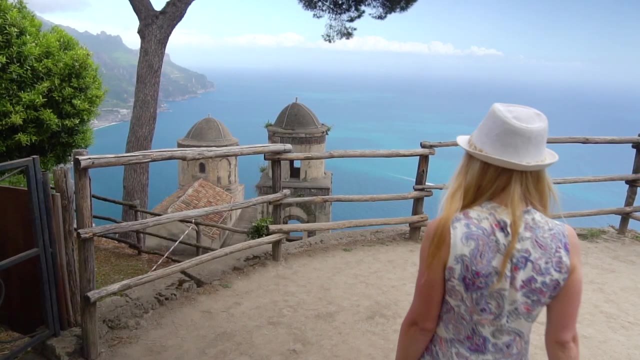 Italy. Spain experiences a similar phenomenon between its industrial north, near Madrid, and its rural south. Among the large southern European countries, France has the strongest economy, powered by telecommunications, shipbuilding and aerospace engineering. But when you think about southwestern Europe, you're likely not dreaming about France's robust. 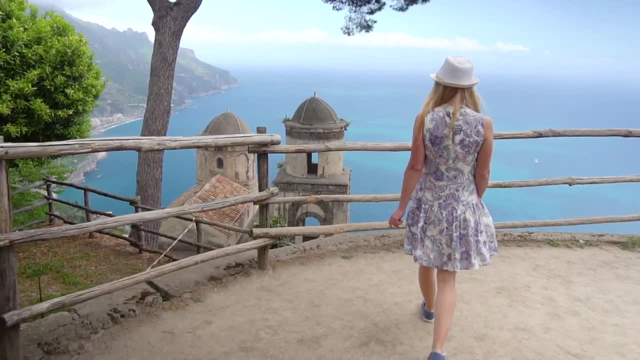 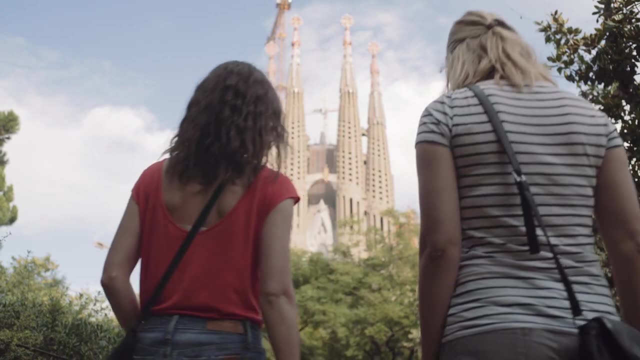 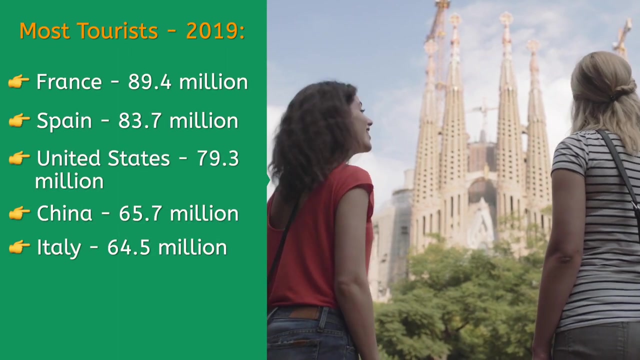 telecommunications industry or Madrid's industrial plants. You want to enjoy the endless beaches, delicious food and the rich culture of the area. And you're not alone. Millions of people each year contribute to the tourism economy of these countries. In 2019, France, Spain and Italy placed first, second and fifth in the world. 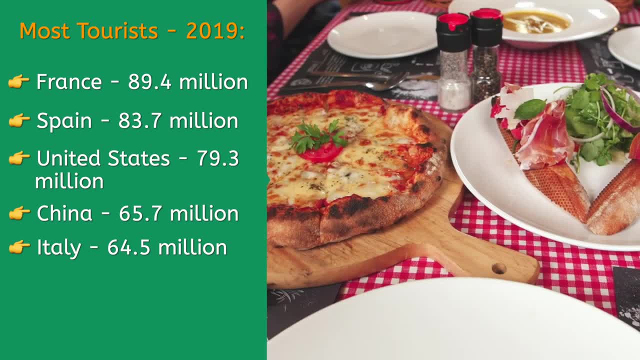 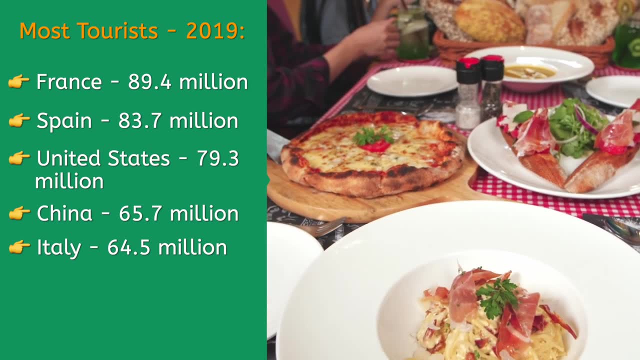 respectively for total visitors. These travelers spend many euros on fine champagne, yamon and lasagna, and that money flows right into the economies of these countries. There are many reasons to visit southwestern Europe, so let's see what else this region has. 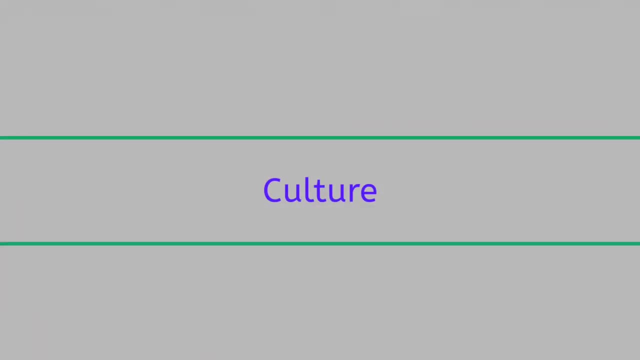 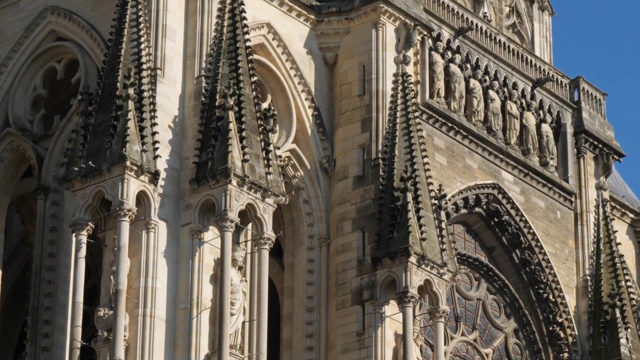 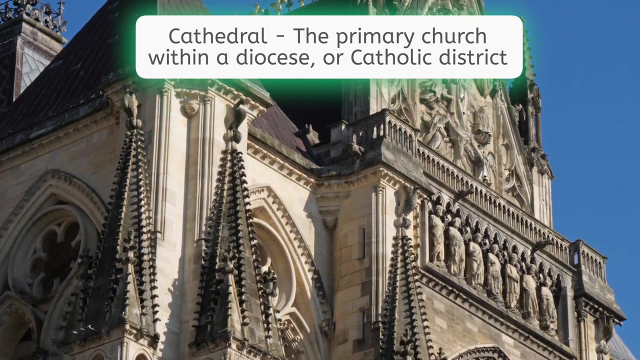 to offer in terms of culture. Culture: Stained glass windows, High vaulted ceilings, Flying buttresses. Where are you? If you guessed an old European church or cathedral, you guessed right. Big city to small village. a church is right there, in the center of nearly every town. 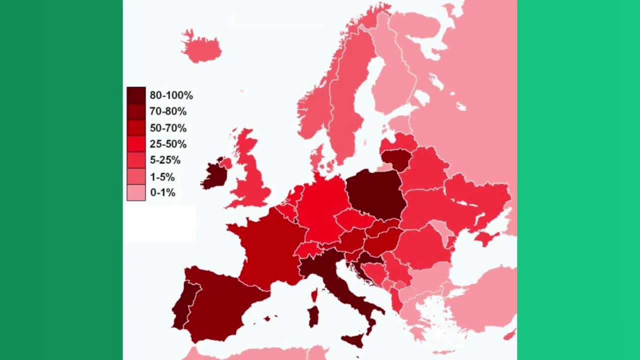 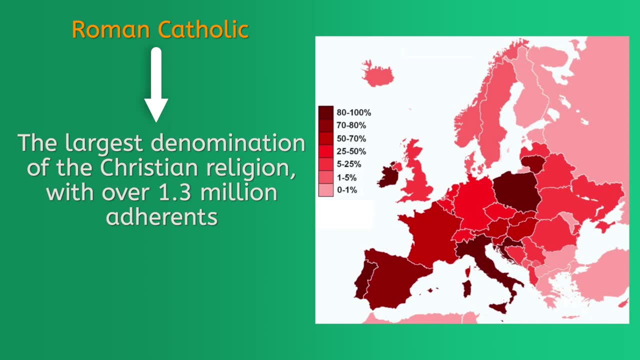 Religion, And there's a reason for that. The region has overwhelmingly been devoted to the Roman Catholic faith for centuries. In 380 CE, the Roman Empire made Catholicism, which is the largest branch of Christianity, the official religion of the empire. Since then, many of these lands have remained. 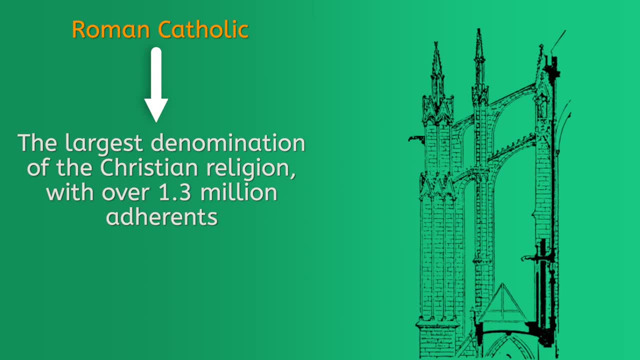 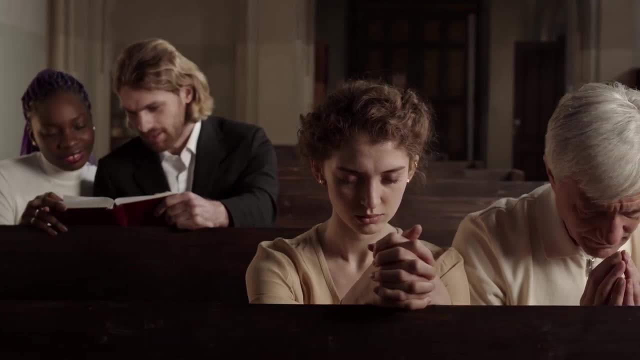 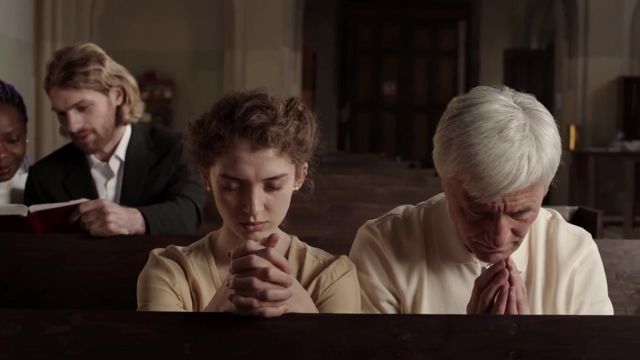 predominantly Catholic. Oh and since I knew you were wondering, no, flying buttresses do not actually fly. Despite this common Catholic thread, religious devotion varies by country. Seventy percent of Italians and Portuguese consider religion an important part of their daily lives, compared to only thirty percent of the French. 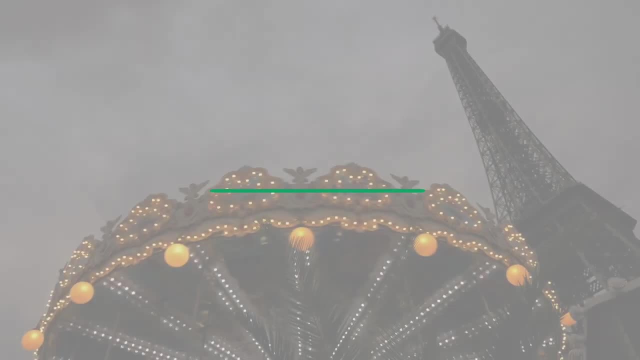 Language Speaking of French. if you've ever heard French spoken aloud, you might think that it's a language of romance. A picnic blanket, A bottle of wine, A glass of wine, A glass of water, A glass of wine? I don't know. 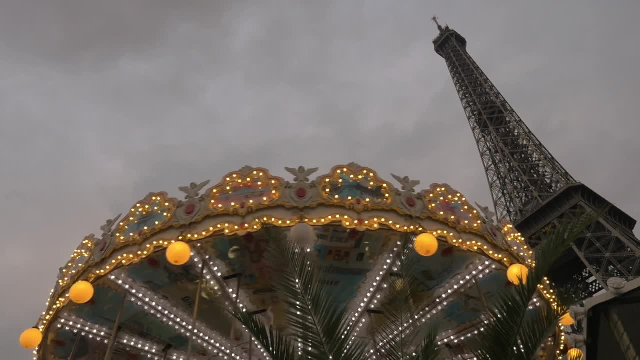 don't you think? But I do. It's a language of romance. A picnic blanket, A bottle of wine, A glass of wine, An Wine, the Eiffel Tower, an accordion player somewhere off in the distance. Je t'adore, mon amour. 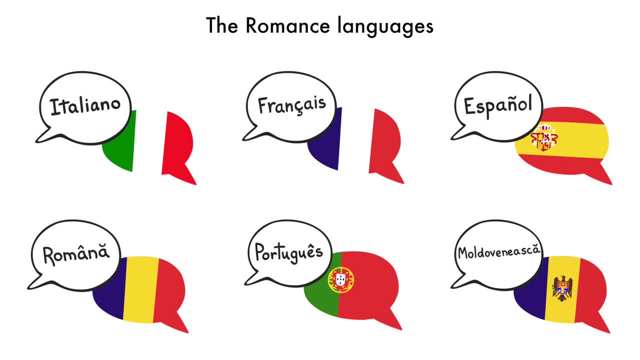 You may be surprised to find out that nearly all of the languages of this region are based on romance, But not the Eiffel Tower picnic blanket kind. The languages of the area are called romance languages because they're derived from Latin, the language of the Roman Empire. 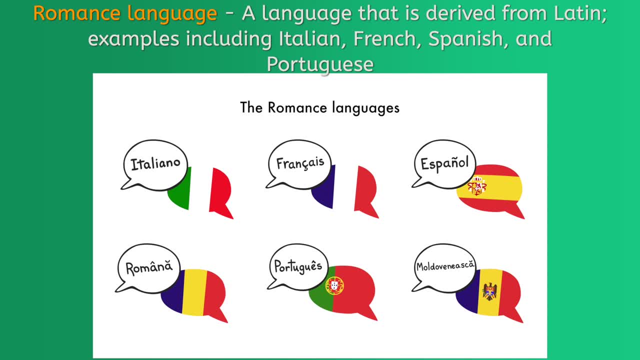 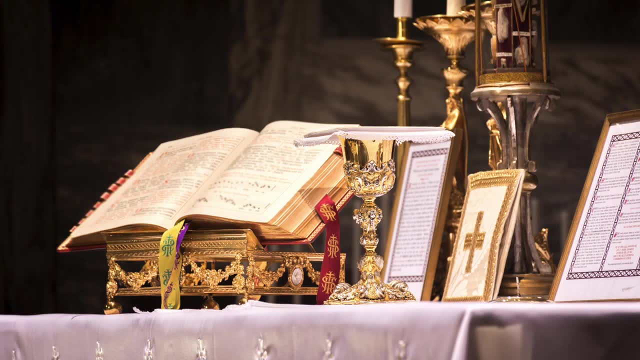 Roman romance: See the connection. Examples of romance languages include Italian, Spanish, French and Portuguese. Now let's tie this all back together to our discussion about religion. For many years, Latin was the only language spoken at Roman Catholic functions. 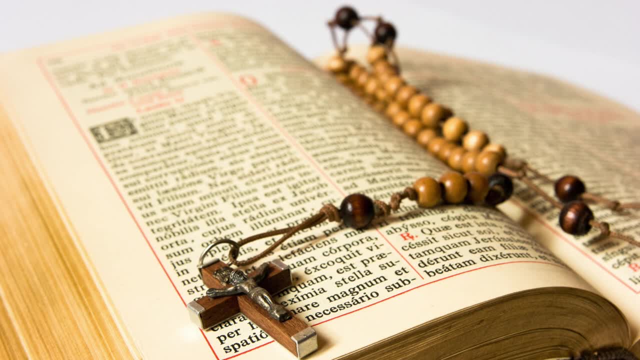 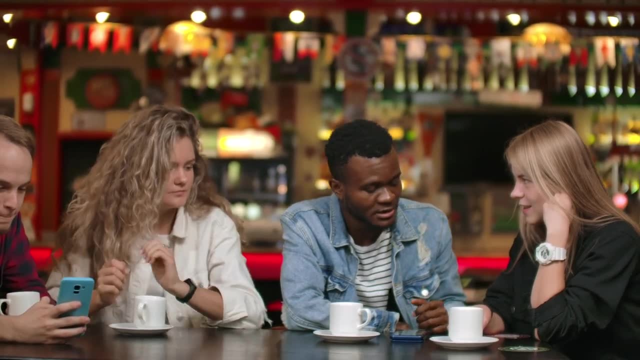 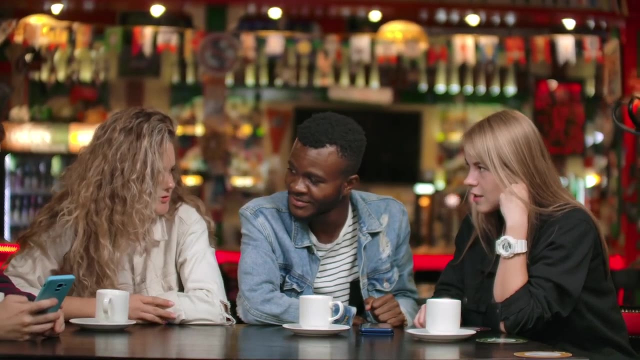 so it makes sense that these Catholic countries would have languages that come from Latin. Additionally, over half of the people in southwestern Europe can also speak conversational English. In general, Europeans consider language learning to be important, so it's only polite to return the favor by learning some basic phrases of the local language. 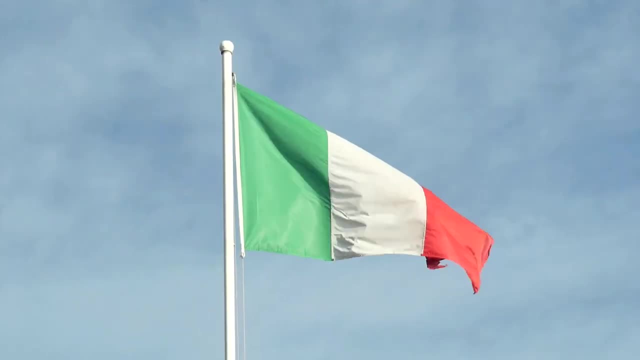 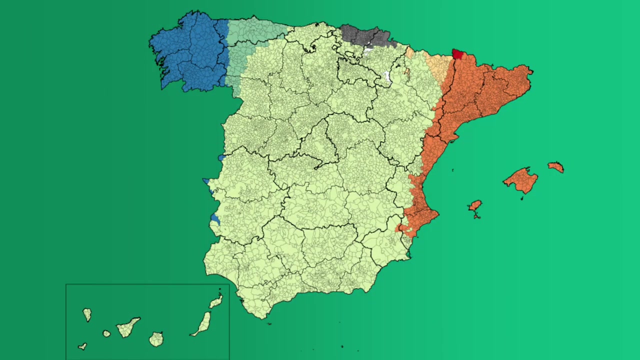 While there are small variations in regional and local culture, most countries' populations are ethnically homogenous. Often, this means that a person's ethnicity matches their nationality. Over 90% of people in Italy are ethnic Italians, for example. There is, however, quite a bit of diversity within the Spaniard population. 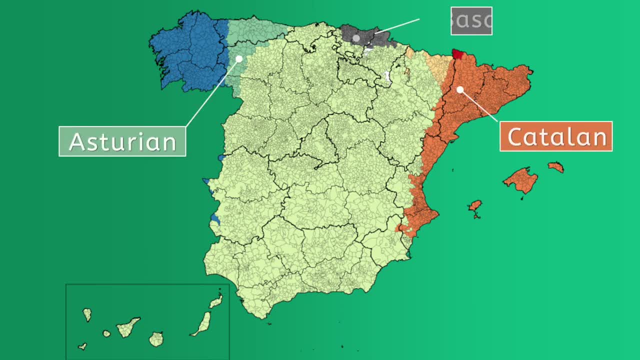 Regional groups such as the Asturians, Catalan, Basque and Galician live in Spain. some Basque and the Catalan have supported independence movements for their land and if you visit, you will encounter different languages, culture and cuisine in each of these regions. 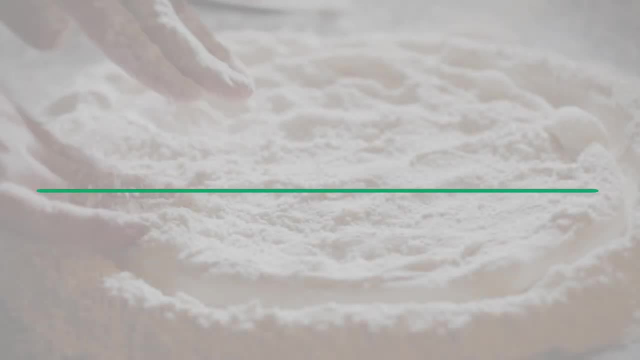 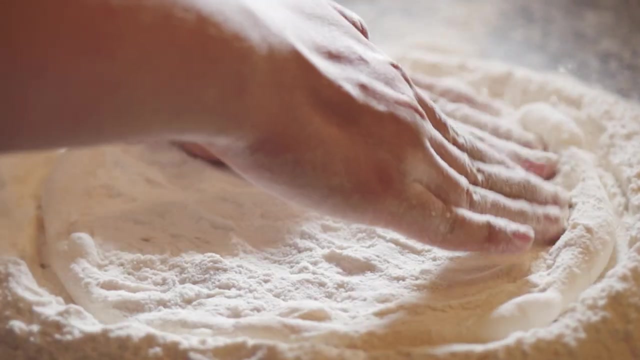 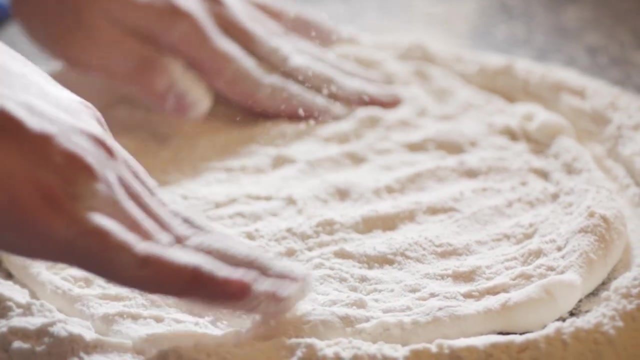 Cuisine. Speaking of cuisine, well, there is one particular cultural contribution from southwestern Europe that many people hold near and dear to their hearts and stomachs, and that's food. In Italy, there's a good chance that you'll need to loosen the belt a bit, because you'll be eating, and eating, and eating. 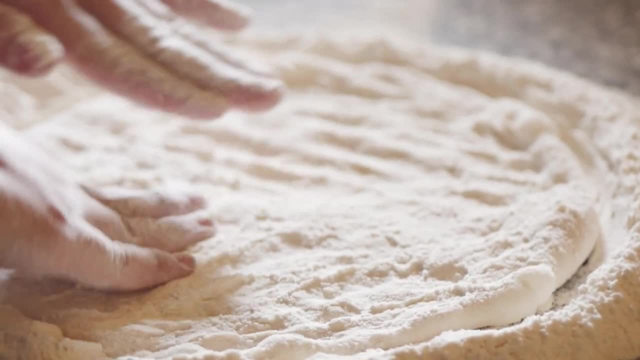 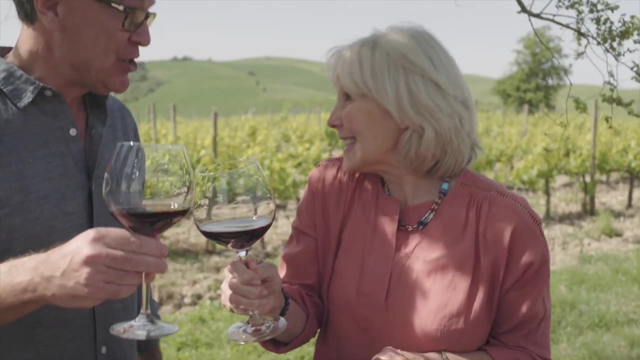 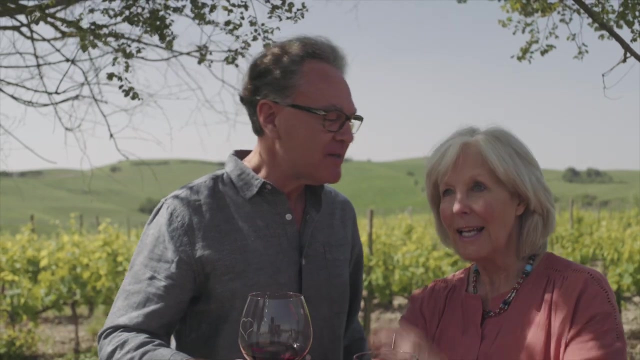 pasta, pizza, seafood- keep it coming. There's a reason why Italian cuisine has been voted by Americans as their favorite foreign food. Additionally, the three top wine-producing countries in the world are located in southwestern Europe: Italy, France and Spain. 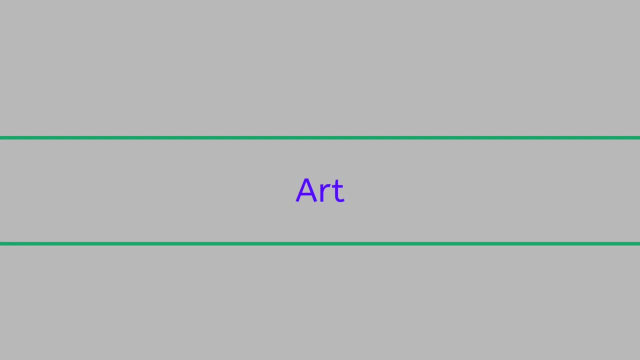 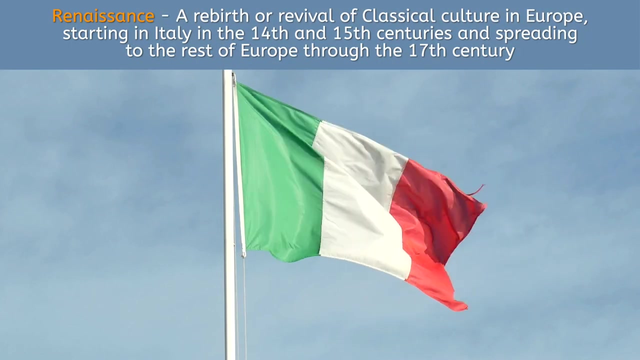